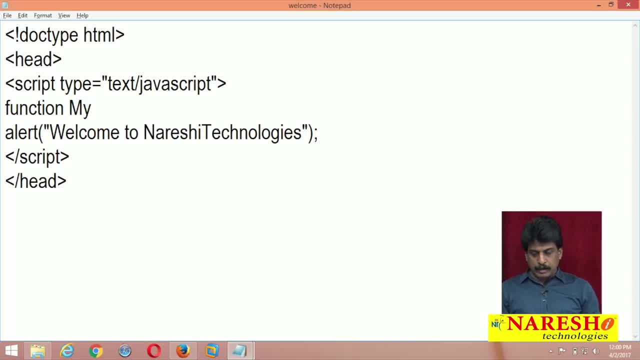 Function: function name. my warning: Yes, function. curly brackets closed. If you are running now, nothing happens Because function is written type You declared but you are not calling. Come to body level. Click the button to display. 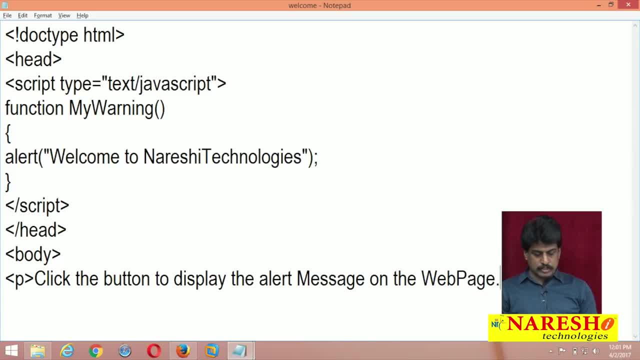 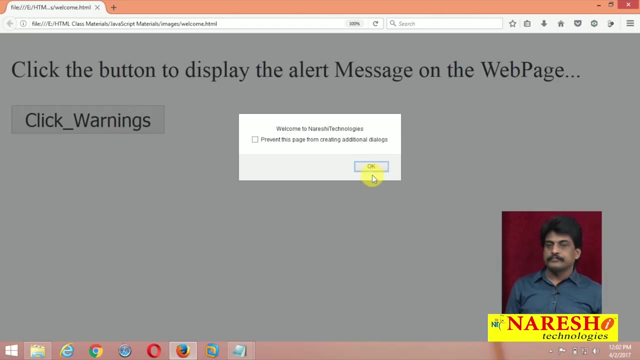 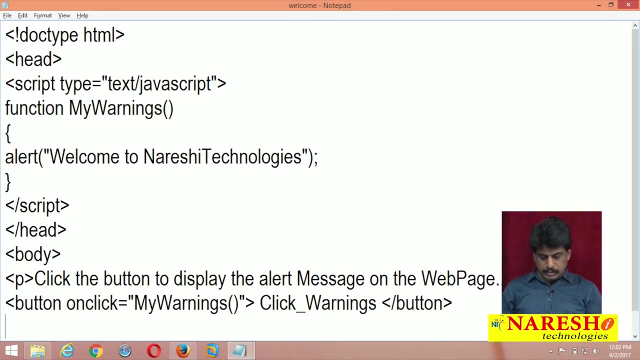 Message on the web page. Button on click is equal to my warning Click underscore. warnings Button close. Just because name I used here, warnings and warnings have changed. Now you can come down, refresh, click on that Perfectly executed. Now, for example, you want to run. I said already five times Yes, simply without going to source code that button. only you can duplicate Refresh it. 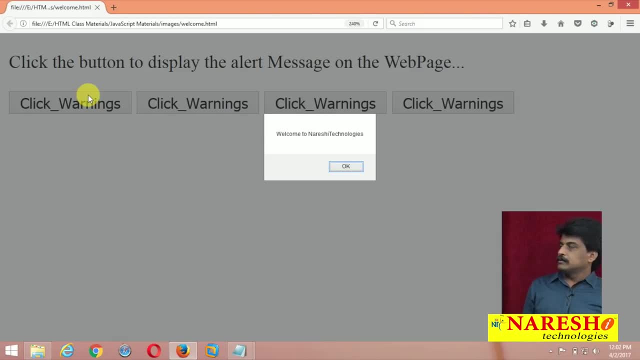 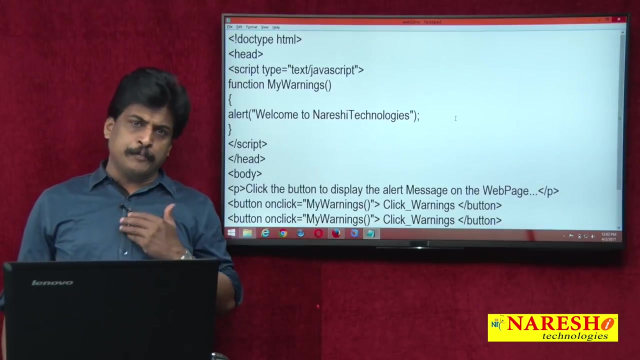 Simple: Click this. You wrote the source code only one time, But how many times you are calling you can observe here. This is called code reusability: Write once and call any number of times. script or any programming language area that declared this part. we are calling as called. 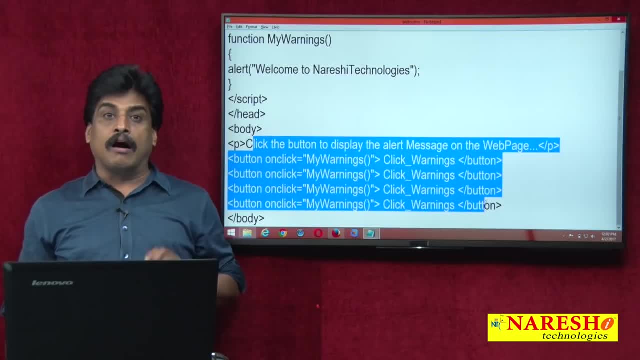 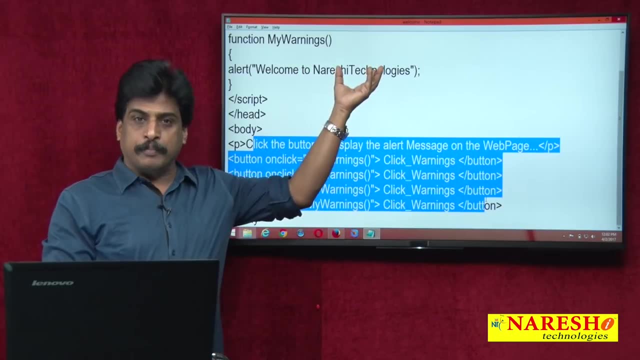 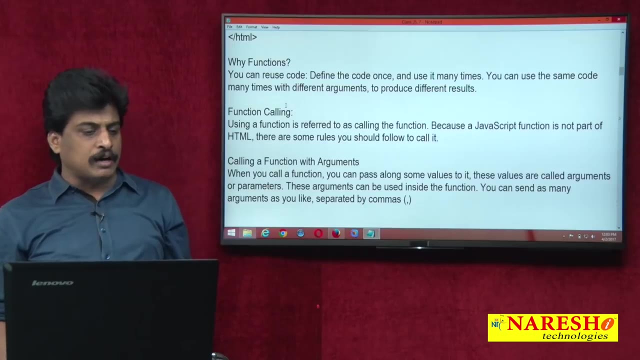 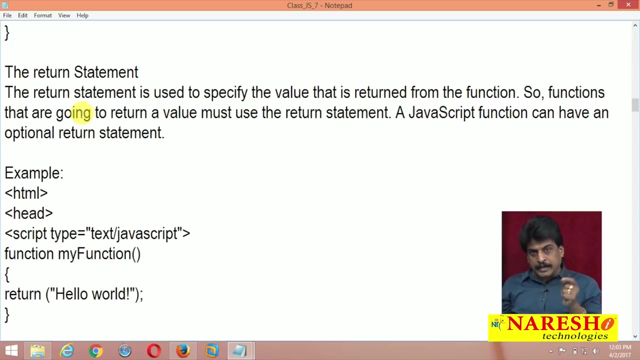 part. This is we are calling as calling part. Actually, we are passing parameters from calling part to called part. That practically we can see, using one written statement, What is actually written in JavaScript. Yes, we can see that A written statement is used to specify the value that is written from the function. 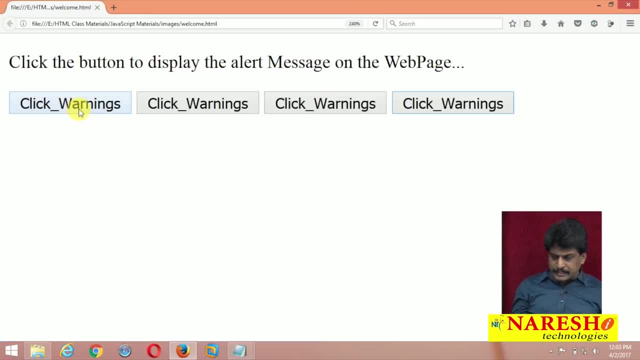 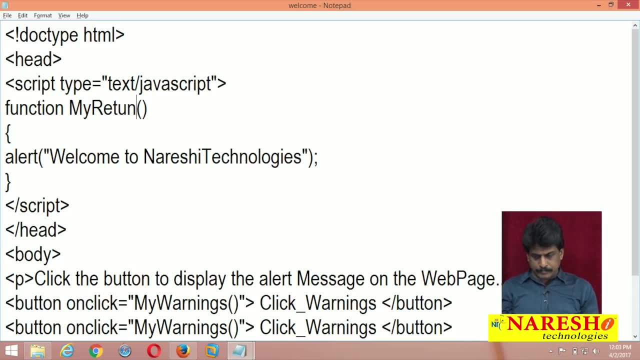 It is always optional statement. Let me develop one written. here Come and we can see my written. Simple: I am writing my written, I am writing written keyword. here I said, for example, hello. I am a written Statement, written keyword. 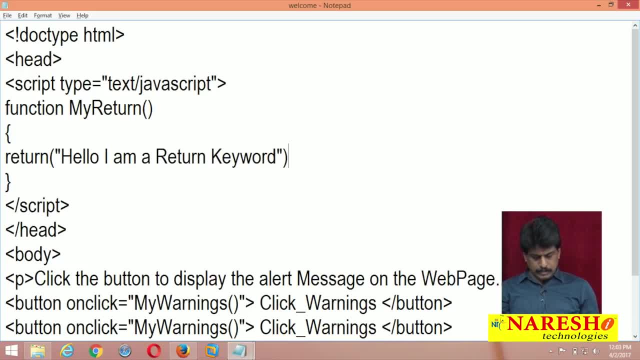 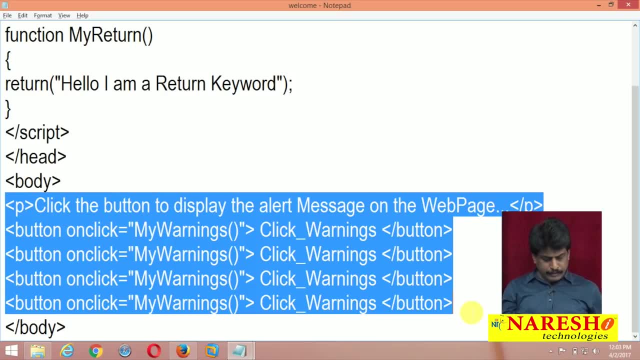 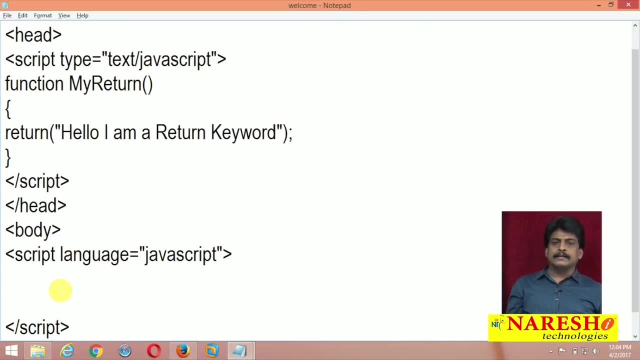 So when I am going to say that written keyword, just close that, and my written is there here. Come down to body section: Little differently. I am writing, Please concentrate. Script language is equal to right Now. I need to write document, dot, write, observe. and what is here? my written. 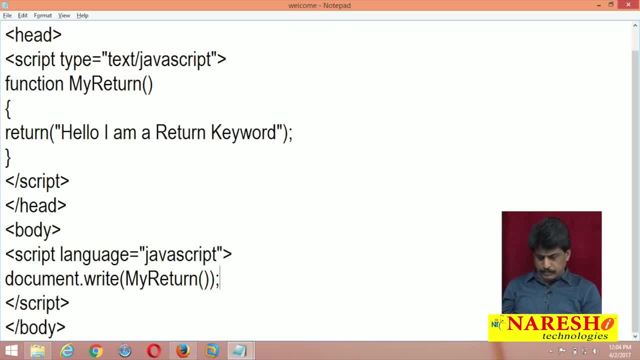 Excellent, Now here you can close and semi-equal. So this is calling part and calling to this one and it is getting executing Really happening that, Okay, come up. So now in the written statement level, whatever existed, yes, simple, I am doing like this: 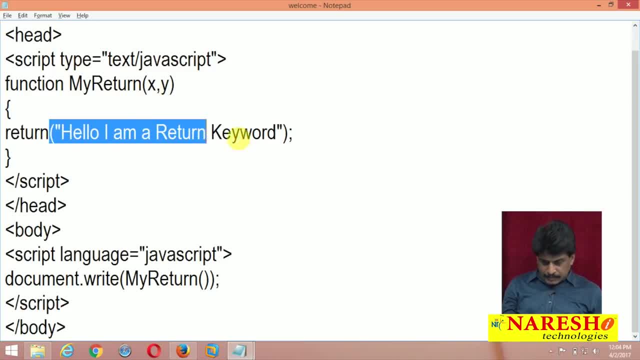 X comma Y. Now I said written written X multiply by Y Means I am doing product. Now I am passing the parameters. For example, 10 comma 10. I am passing These are the parameters. These are the arguments I am passing. 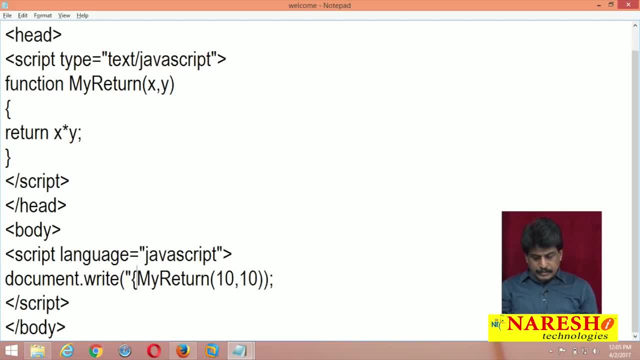 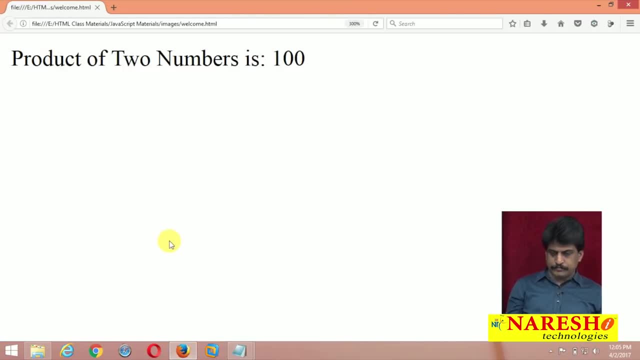 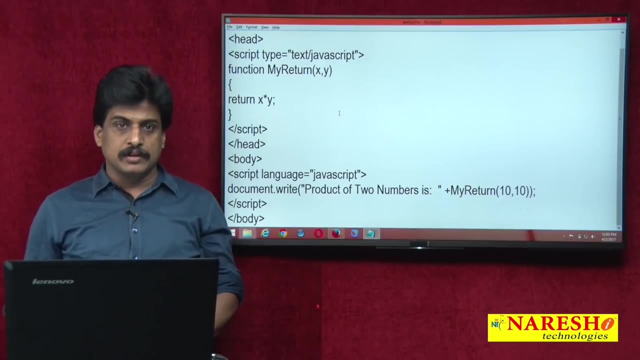 Now, for example I am giving here, product of two numbers is, and now refresh, So perfectly displayed. This is called passing arguments, Passing parameters, The called part. this is Calling part. is this one? Now simple? I want to write the point here. 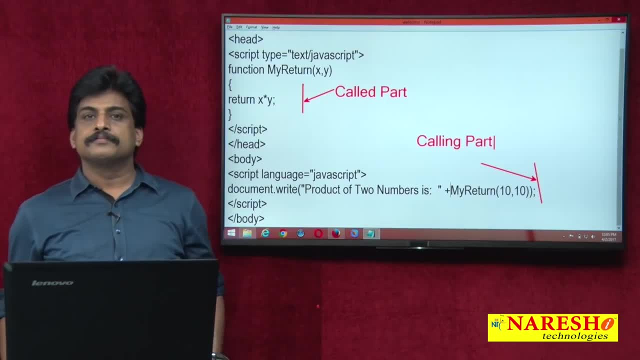 Called part: Calling part. So parameters always available in the calling area, Arguments always available in the called part. This is the body of the function. So now you can declare in the script area and you can call from the script area. 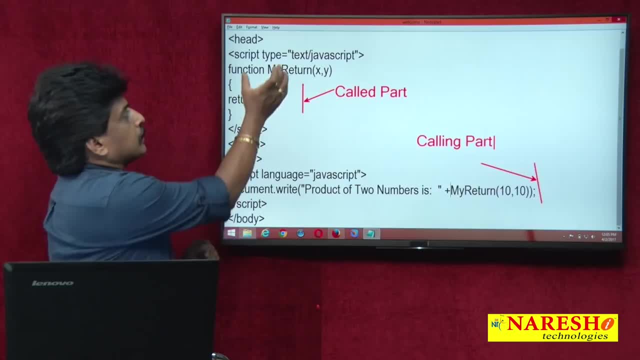 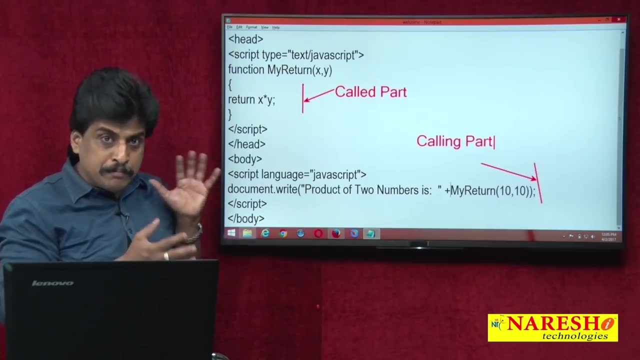 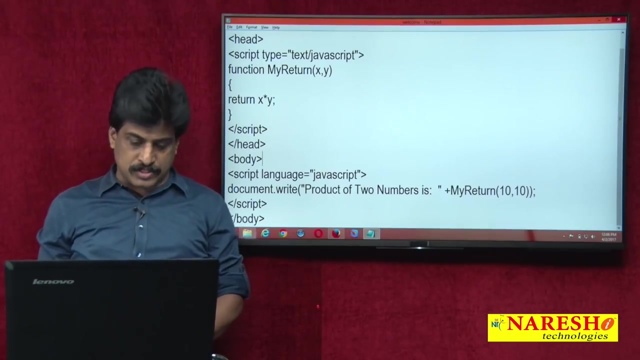 But there is no rule here: Language must be written and time must be written like that rule is not there. The type attribute you can write here. Language attribute: you can write here. Very basics, fundamentals. Now, once you pass that lifetime of JavaScript, variables are existed. 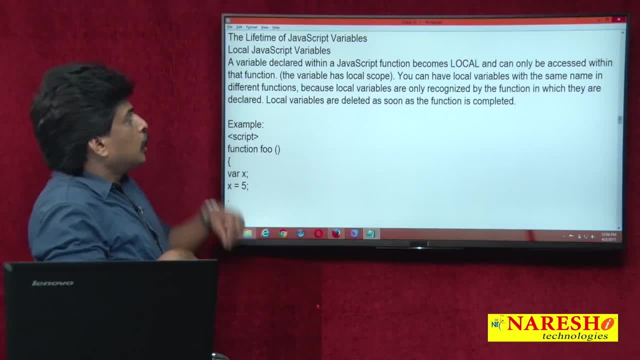 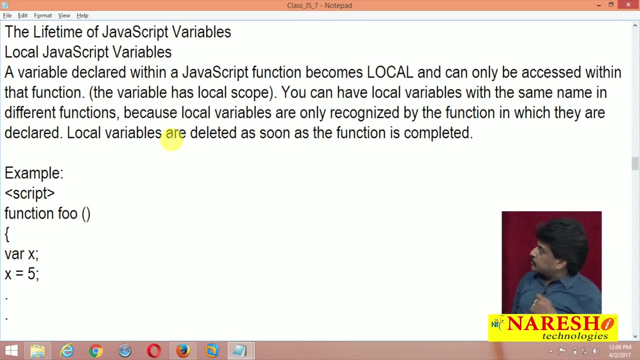 What is the meaning of lifetime of JavaScript variables- Local JavaScript variables, global JavaScript variables- Within the function. if you declare a variable that is comes under local JavaScript variable. I wrote very clear the definition: A variable declared Within a JavaScript function becomes local. 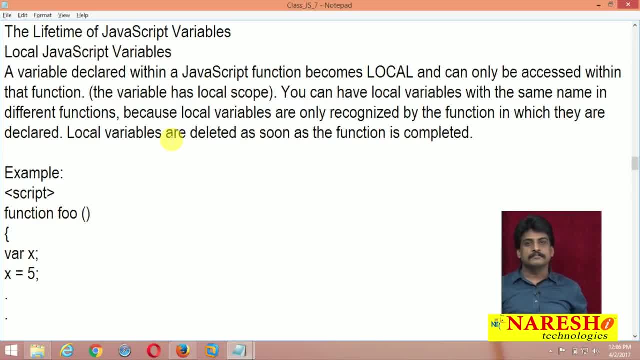 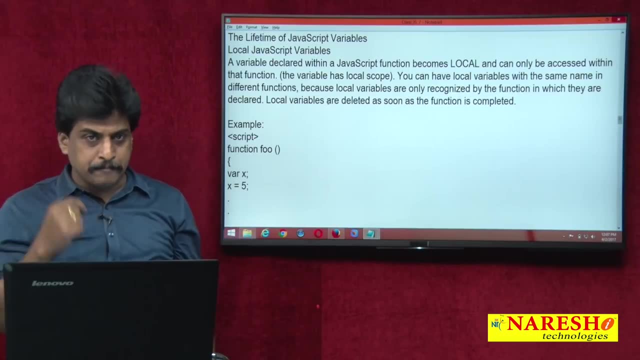 And can only be accessed within that function. Within that function. Okay, The variable has local scope. You can have local variables with the same name in different functions, For example function 1, function 2, function 3.. I declared in the function 1, where variable A: 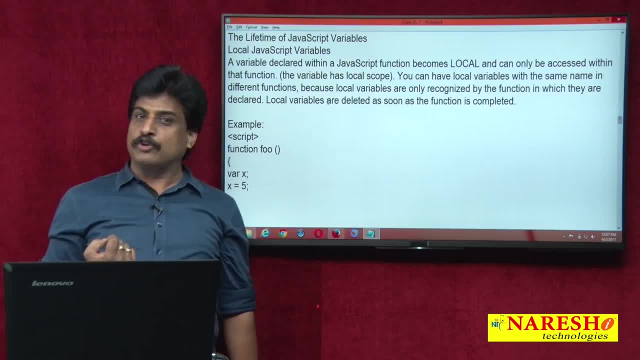 Where variable B Again, where variable A You can declare once again, No issue Means: once you declared one variable within the function, Its scope always local Within the function must not be duplicate. Out of that any number of times we can duplicate. 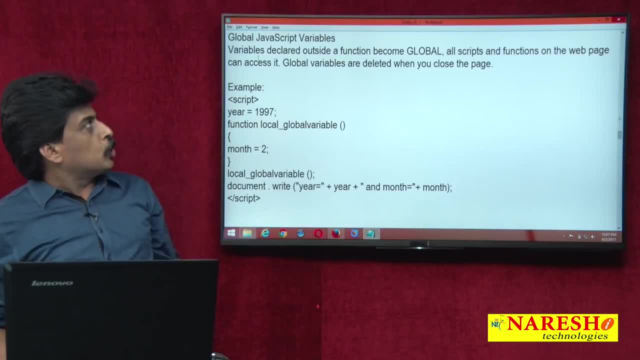 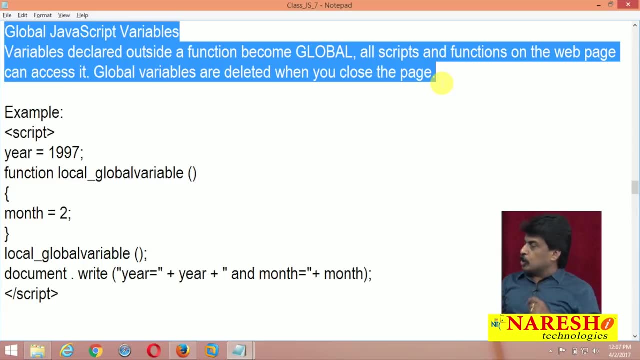 A small example we can view And let me show global JavaScript variables definition. also Observe correctly. Variables declared outside a function become global. All scripts and functions on the web page can access it. Global variables are deleted when you close the web page. 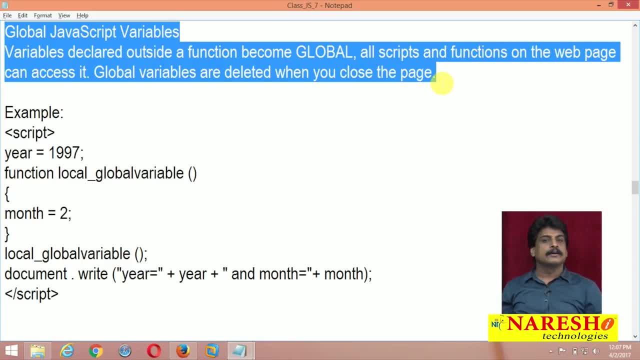 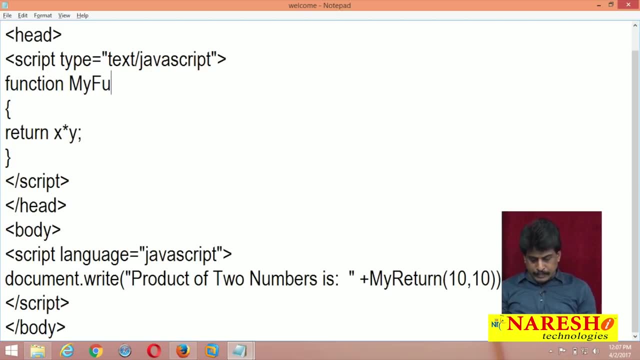 When localized Local variables are going to be Means when you close the curly bracket. Now we can observe practically that. Now, for example, I declared my function 1.. My function 1.. Simply, I said like this: 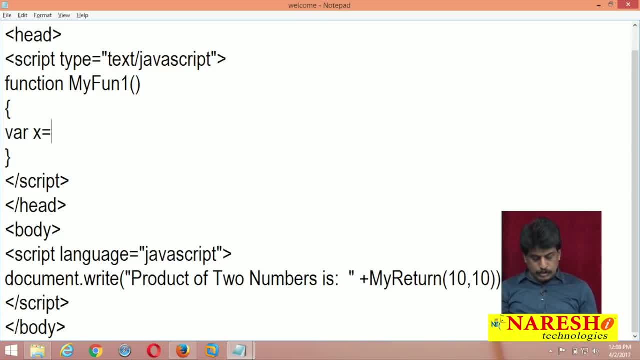 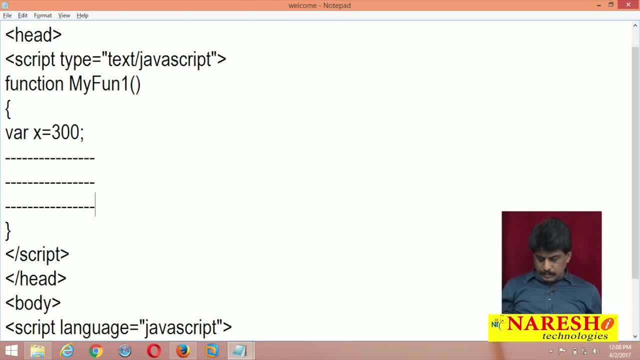 And I made inside where x is equal to 300.. Now some statements. I am writing Some line of code: Write: implement that. Okay, good, One function completed. Before the function I said Where a is equal to 400.. 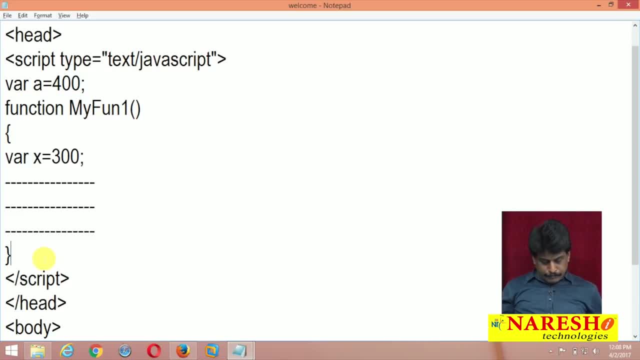 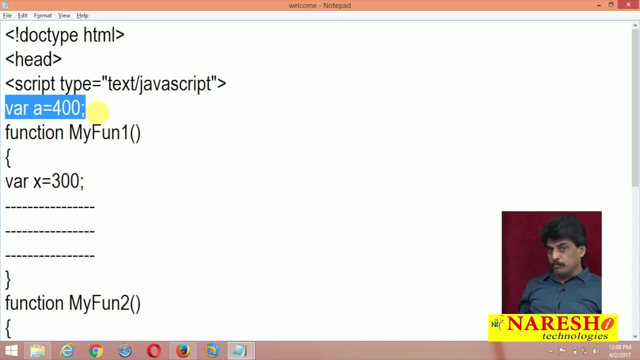 Now, inside the function Write another function. I am implemented Two functions: Function 2. And I said here, where y is equal to, I said 400.. Them statement, So observe here: A comes under global variable, Global JavaScript variable. 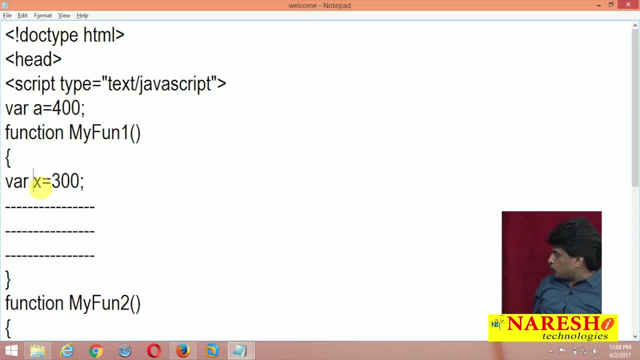 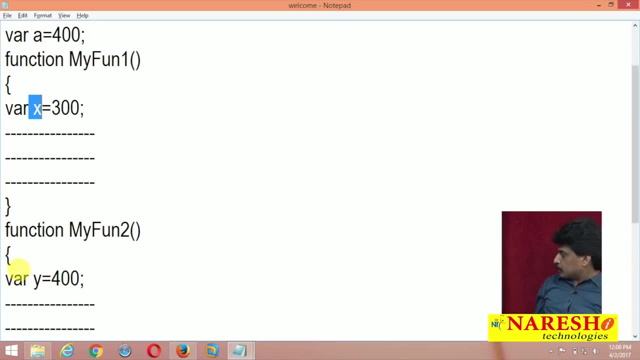 And x comes under local JavaScript variable. Its scope is max here. Once this part completed, X will be deleted. Died Simple, I can say: Now again, y is there. So this is also local scope Up to here available. 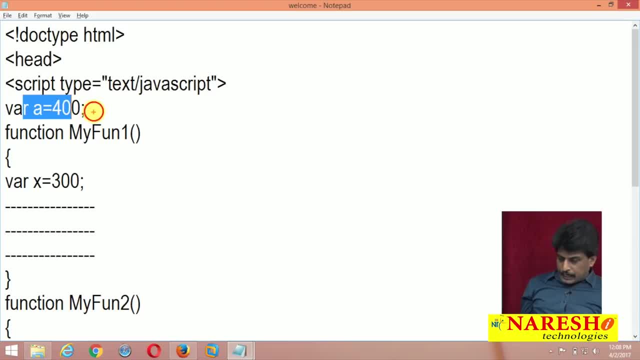 But this, a variable scope Applicable to And x, means this function level And this function level. That is the reason. If another function available Or another procedure available, It is global. It is web page level. The point I made very clearly. 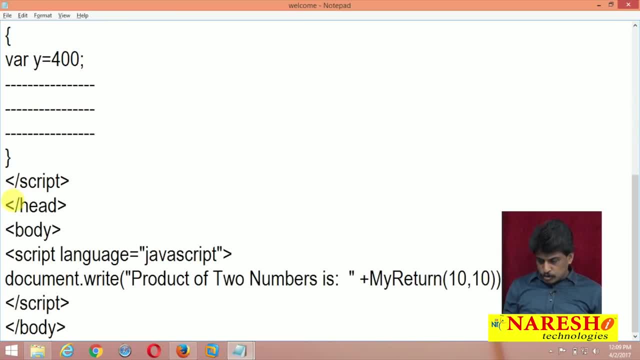 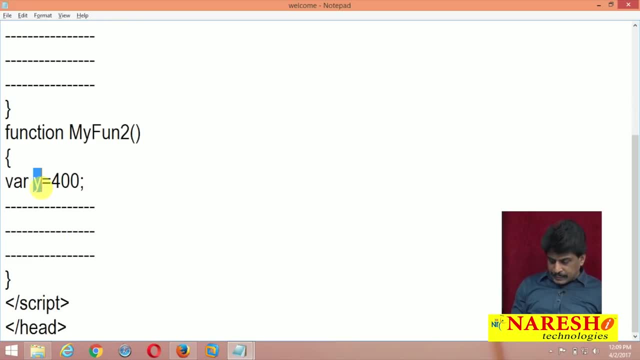 Just a few minutes back Now, for example, Close it all The three, The things I am going to be delete. this Right Observe. So now X again. I am duplicating, Duplicate, no problem Here. x available. 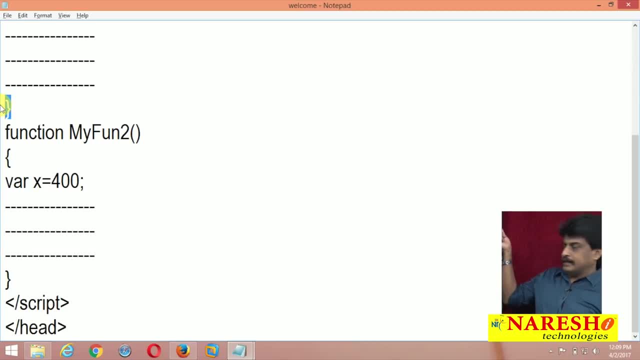 Here x available, No problem, Because scope is here. Closed Here. only deleting Here. if you are using that, There is a thing happens. For example, a is here. That a, for example I am using, Must not be. Global variables are unique. 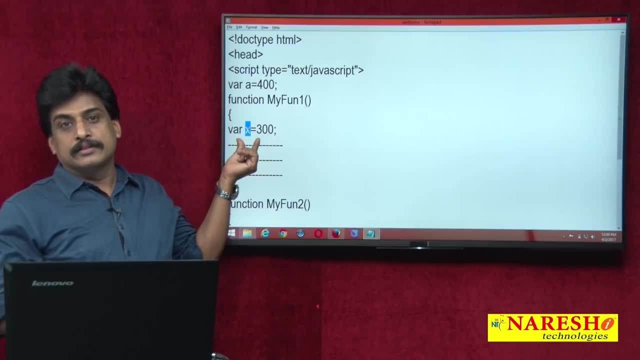 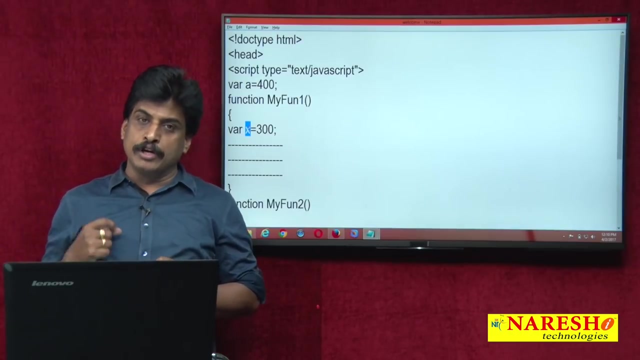 So you should be only other than global. So this is about Your variable scope In our java script. Let me move to one Method is there here Inside the document object? Using that method, We can able to change the background colors of the web page. 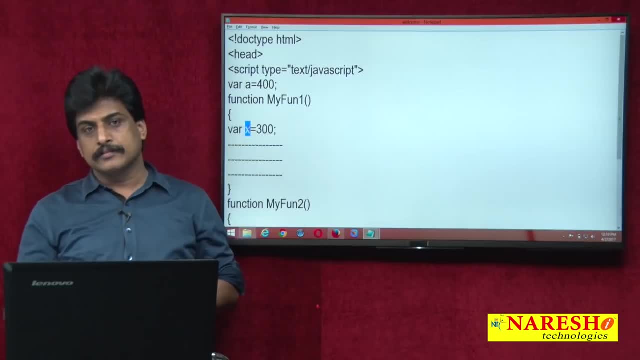 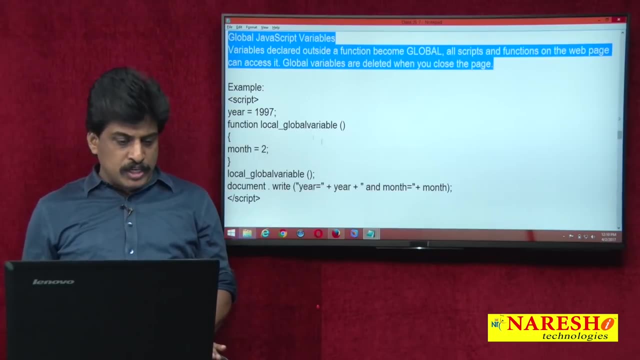 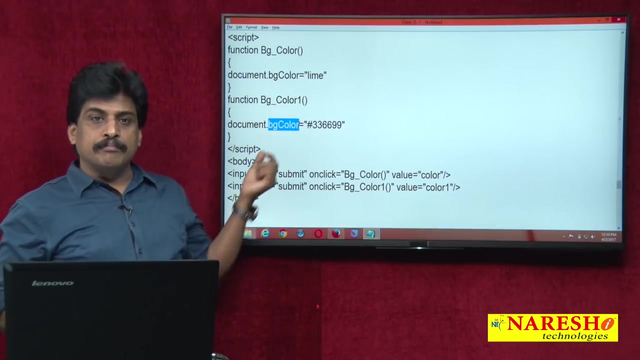 Document: dot. bg color. Using this property, I can say not method This property. you bg. Bg color property. We can change background color. This is the background colors- Bg color property. Background color of the web page. Let me develop simply that one. 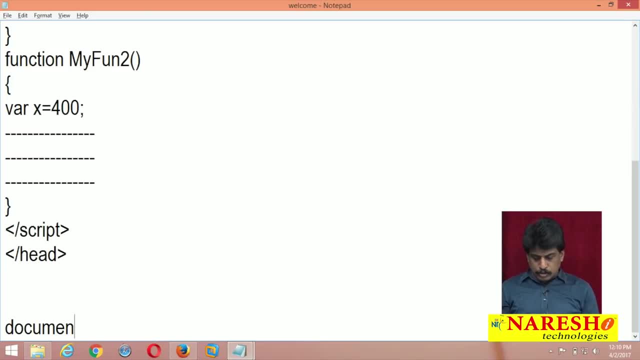 The syntax. let me show first What is the syntax of that Document. dot bg color is equal to color name or color code. Color code means x or a small color code we are writing. So of course, in previous video sessions I made very clearly. 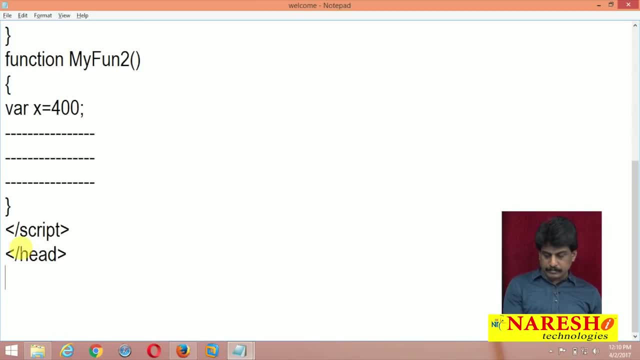 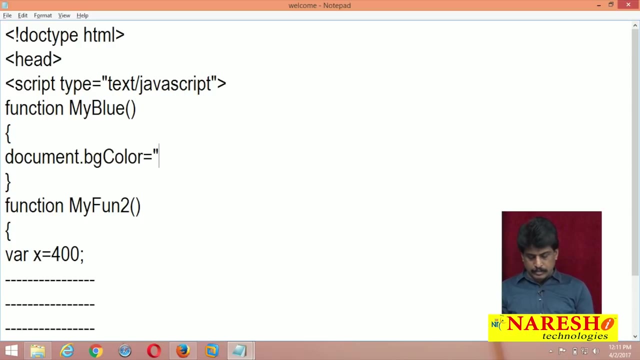 Each and every color code Right. Let me develop A simple example. So, for example, I am coming to function. I said color name is my blue. Now I am writing here: Document dot bg color is equal to hash 00 and 00 ff. 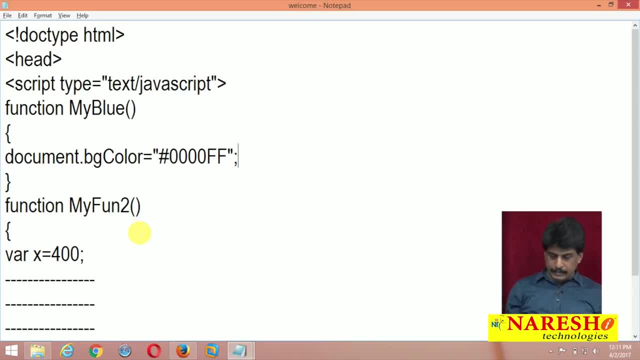 Red, 0 green, 0 blue- And I am coming to my blue- Only the function. I am writing right now. I am not writing any other thing. Right, Come to body, Body level And body And paragraph On click is equal to.